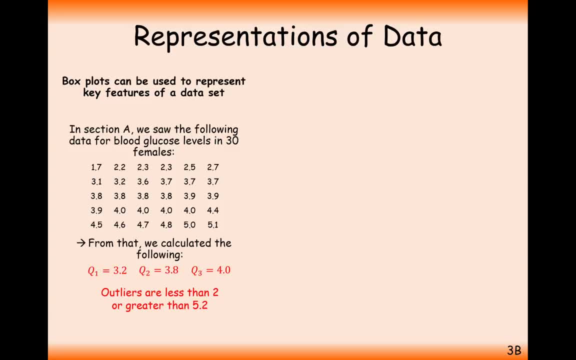 So outliers were 2 and 5.2. Outliers were less than 2 and greater than 5.2. So represent this on a box plot. So what we would do first is put a little marker at the smallest value. that was. 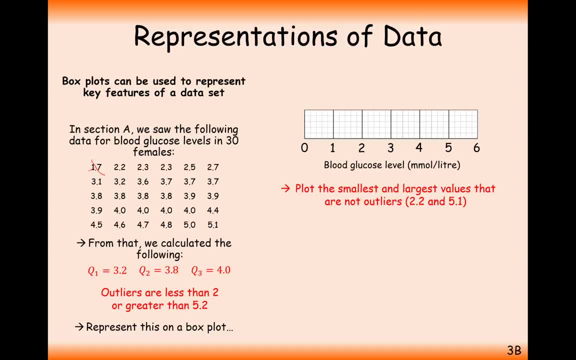 not outliers. So we knew that the outlier for 1.7 was an outlier. so the next value for now is 2.2.. So we'll put a marker there and a marker at 5.1, which was the highest value Markers at the quarter waypoints, and then we'll just connect all. 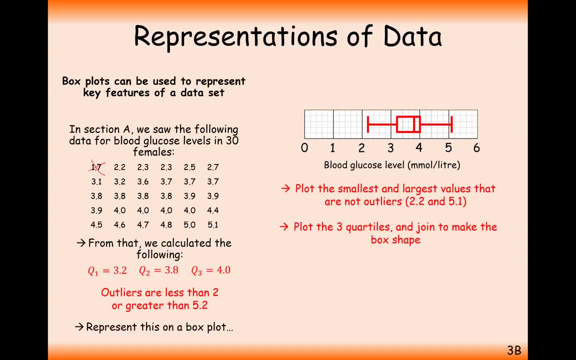 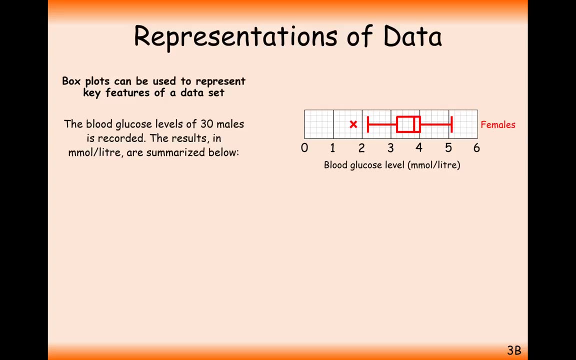 those up, making a box with three middle points and then whiskers effectively out to the lowest and highest value and then put a little cross at the outlier. Okay, so that's a really basic way of drawing a box plot diagram and indeed they are a basic topic within A-level maths. 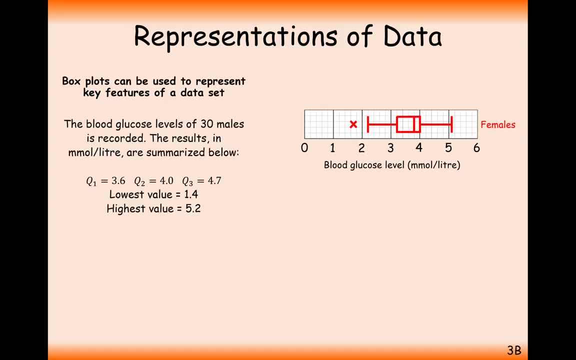 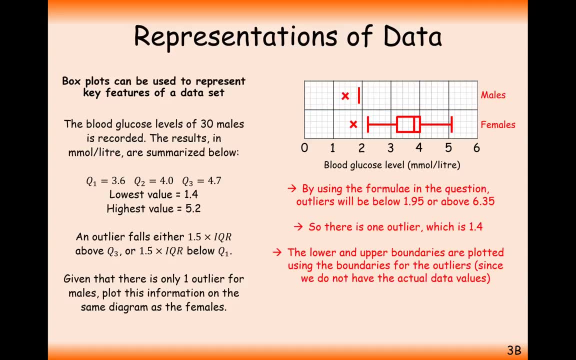 So another set of data gives us blood glucose levels for males, and they give us this data here. So plot that. So let's have a look at how we can compare data using a box plot diagram. Now here we knew that the lowest value was 1.4 and the highest value was 5.2.. We could 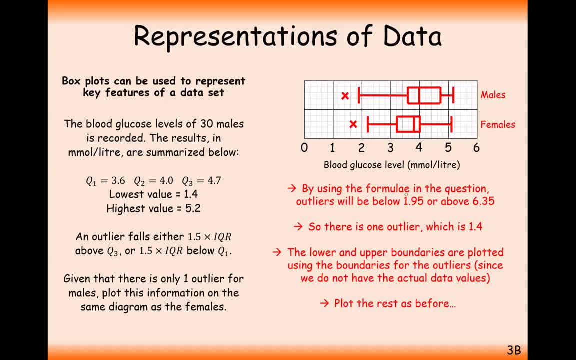 work out here that the outliers were from 1.95 up to 6.35 and anything outside that range would be an outlier. Now, given that 1.4, the lowest value would be outside of this range of exceptions, So that's 1.4 and the lowest value would be outside of this range of exceptions. So 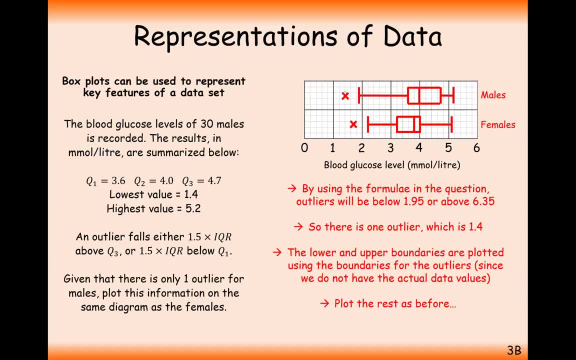 the first answer we need to get out of this is clearly 1.4, and the highest value would be from 5.2.. So that's 1.4 and because we don't know what the next lowest value is going to be, we don't. 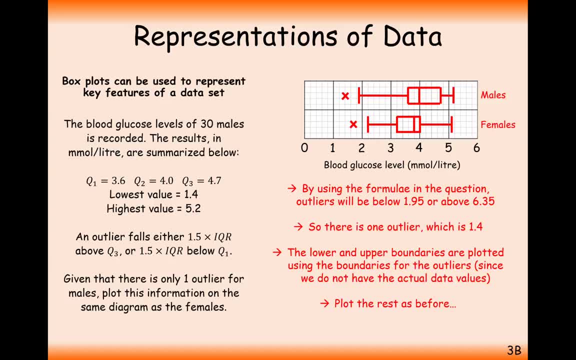 know it will be 1.96,, we don't know if it'd be 2, we put a line at 1.95.. So if we don't know the next highest piece of data from those outliers, then we put the marker at the outlier. 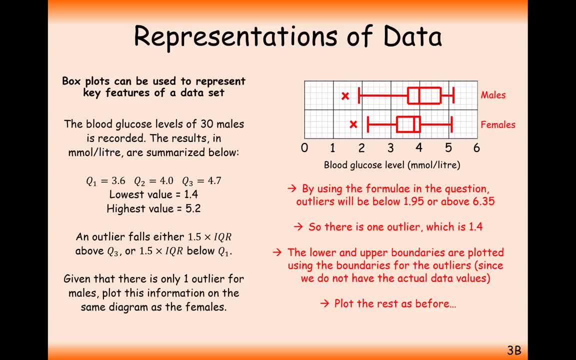 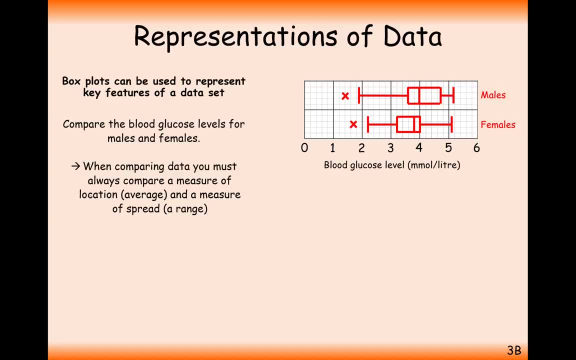 mark, just like we've done with the males here. All right, then. so now we can compare our set of data. Now, what we can say here is: we're going to compare the data in two different ways: the average and the spread of our data. 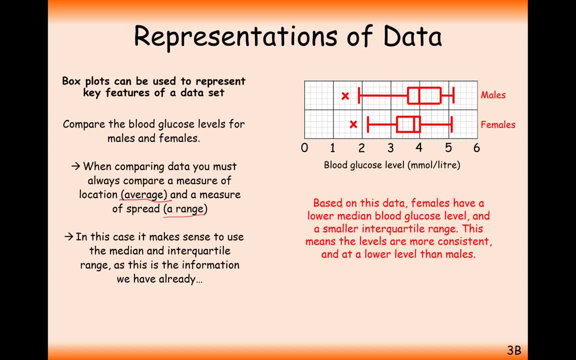 So what we can say here is that, based on this data, females have a lower median blood glucose level and a smaller interquartile range. This means that the levels are more consistent and at a lower level than males. So what it's done there is: it's compared the median out of our set of data and the interquartile range out of our set of data. 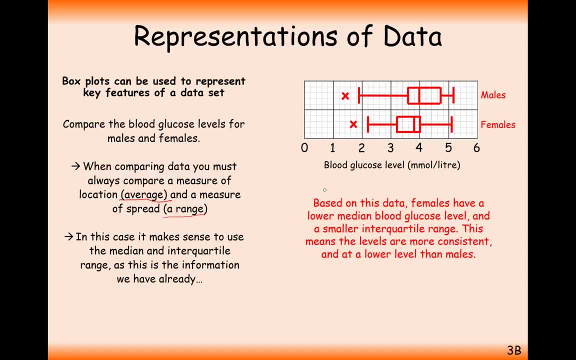 and then translated it back to what the question was looking at. It says that because of the lower interquartile range, it was more consistent and had a lower level than males in terms of blood glucose. So it's really important that you compare the median. 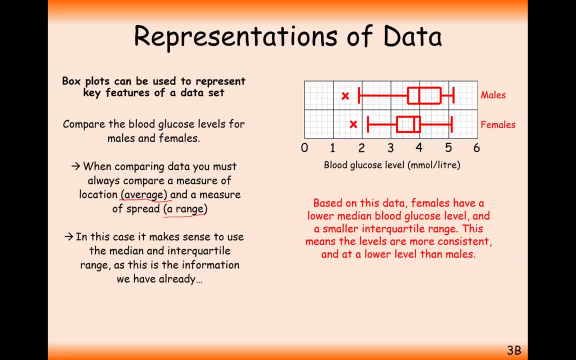 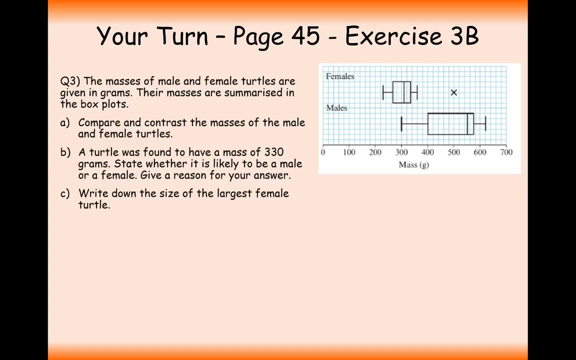 You compare the range, The spread of data, by the interquartile range, and then you link it back to the original context of the question, And it's always used like that. Right then. so have a go yourself. then Pause the video and try this question out. 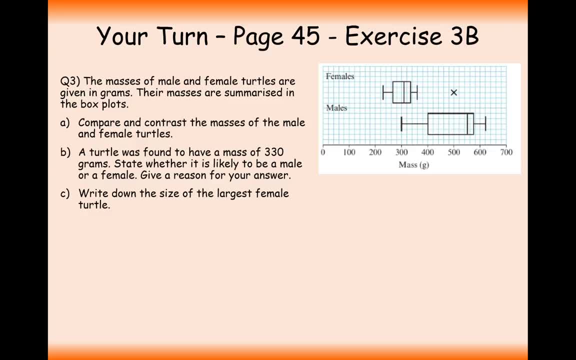 All right then. so here we have a question about the masses of male and female blood glucose levels. Here you can see that the weight mentioned here is actually a greater than or equal to thesover of the male-female turtles are given in grams. 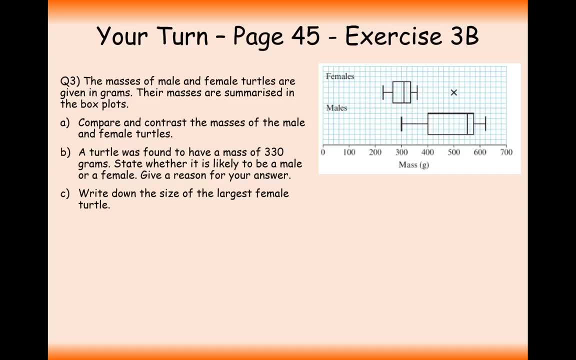 Their masses are summarized on in the box. plots Compare and contrast the masses of the male and female err turtles. So what we can say here is that the median err weight of male turtles is greater than females, showing that they are on average heavier. so that's comparing the 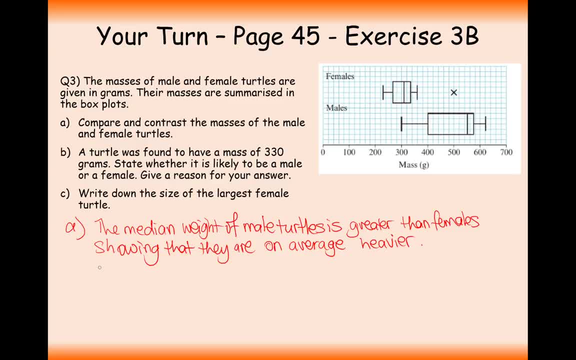 medians and then we can say that the female interquartile range- and you can write IQR- that is a standard notation for interquartile range- the female interquartile range is smaller. therefore females have a more consistent weight. 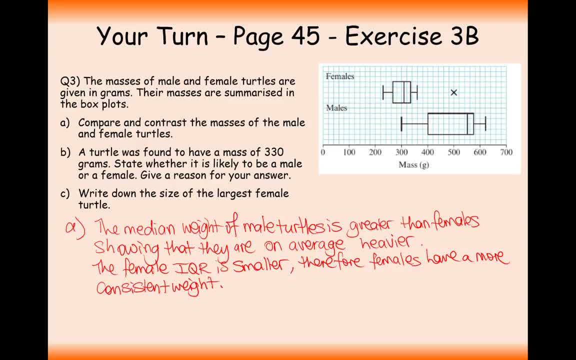 Okay, so that is how we would compare the weights of turtles there. we wouldn't even dream of doing that, comparing weights with human beings, obviously. Okay, moving on to part B, a turtle was found to have a mass of 330 grams. states whether 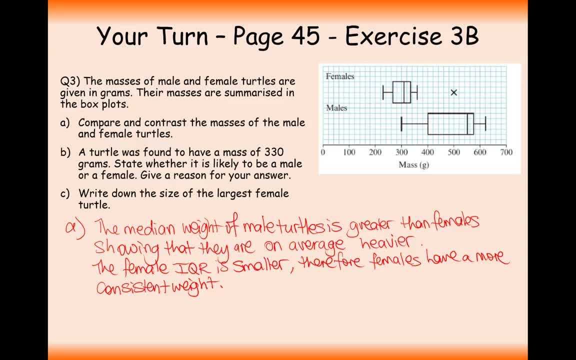 it is likely to be a male or female, Given a reason for your answer. So it has a weight of 330, so that's a little marker at this point here. Okay, I would say that, having looked at this data here, that because 25% of the female data, 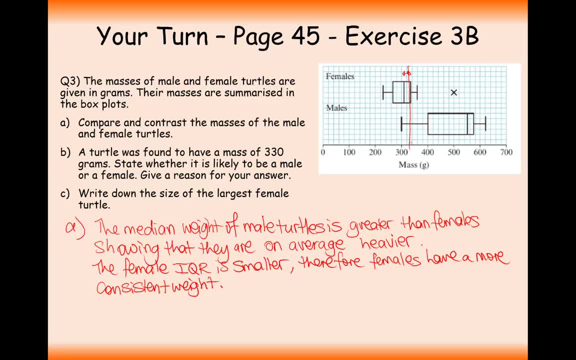 is in this very small mark that contains 330, there's a higher probability that it's in this very small region of the diagram here, rather than the 25% of data that's in the very large region here. So I would definitely say female, as 25% of females have a weight in between. now what 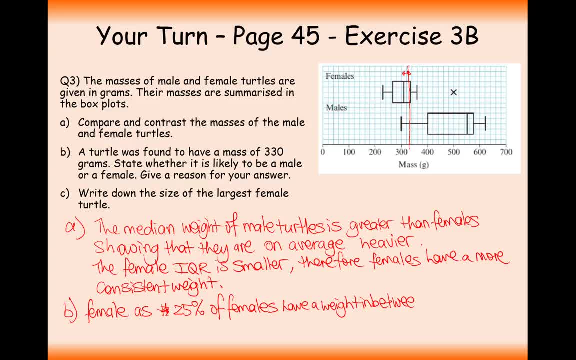 we're assuming here in this answer is that we're assuming that the female data is in this very large region here, rather than the 25% of data that's in the very large region here. So I would assume that we have the same amount of males and females has a weight in between. 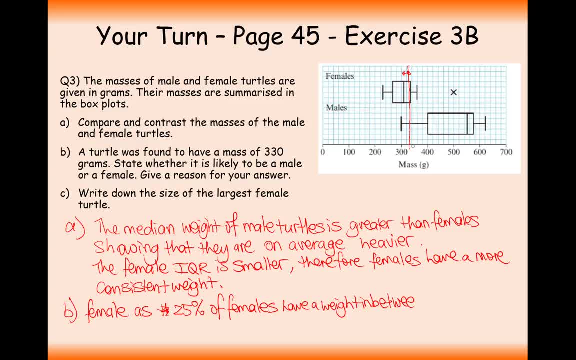 305 and 318.. Between 305 and 308.. Now, with these sorts of questions here, if I've read the diagram ever so slightly wrong, then the invigilator will give me benefit of the doubt and will give me a little range.